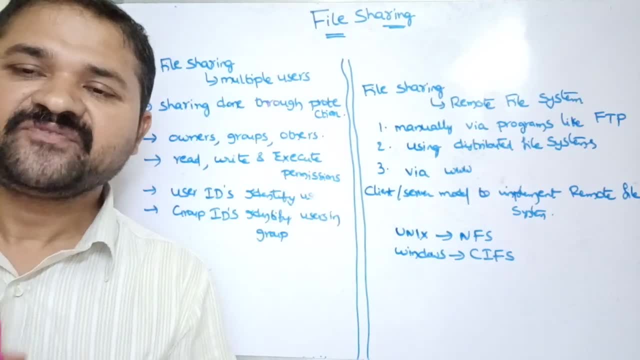 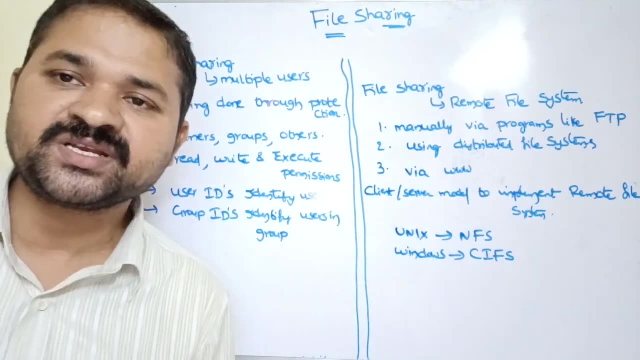 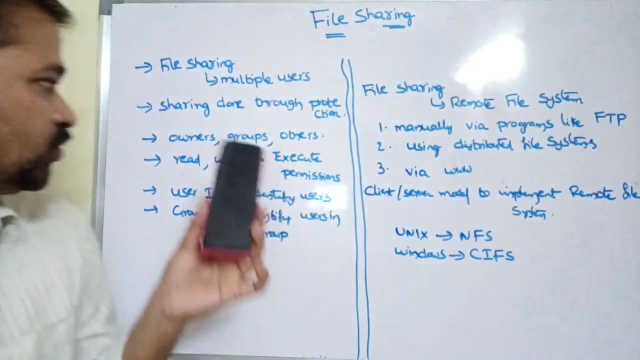 Now let's see about file sharing. We can share file among multiple users, but here there is a problem that other unknown person may access our file. So we have to provide some protection mechanism to our file. So here sharing is done through a protection mechanism, then only other. 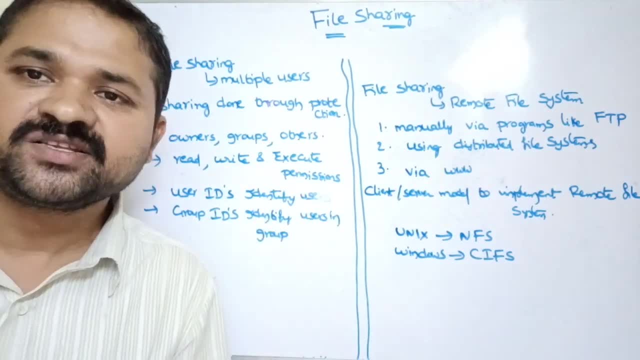 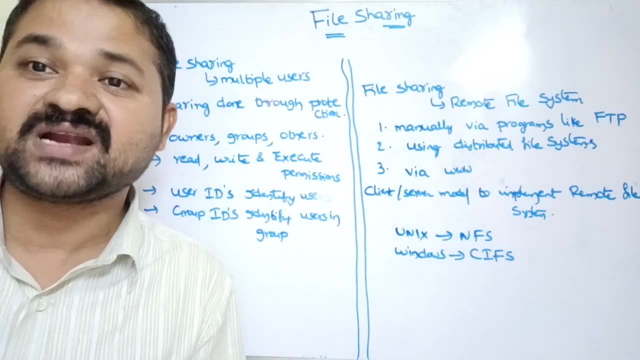 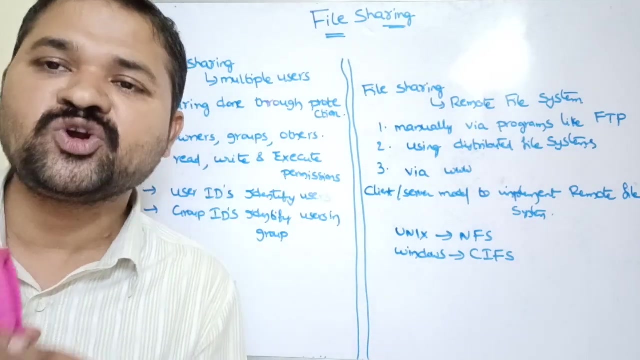 persons cannot access our data Here. in order to provide the sharing, we use the concept of owners, groups and others. So that is nothing but Linux permissions. We know that we can have three types of permissions: Read permission, write permission and execute permission. A owner has the. 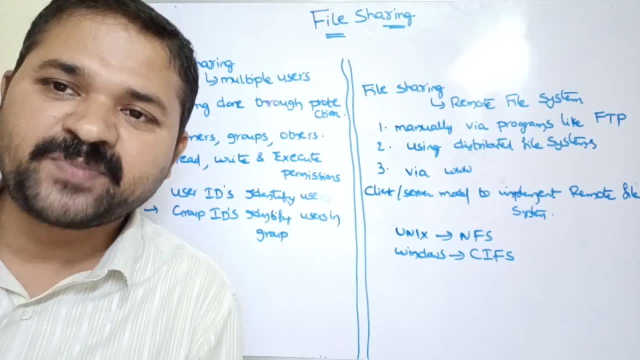 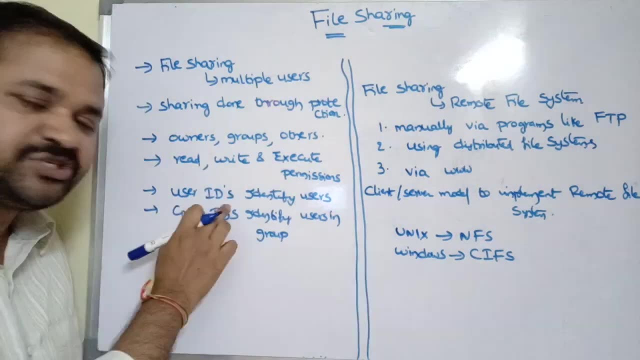 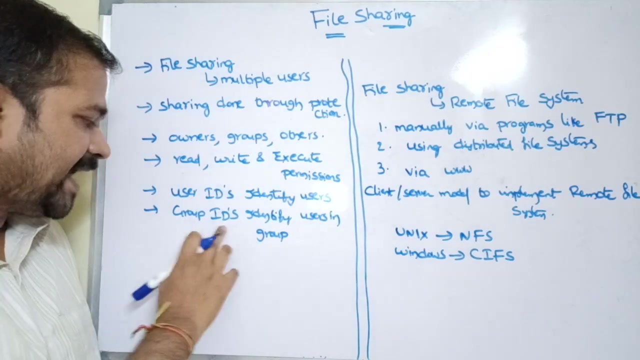 responsibility of allocating and changing the permissions to users, group members and others Others here we can have. for each user we can have some user id, as well as for the members who are in group. They have group ids. so whenever a request comes from an user id, then operating system will. 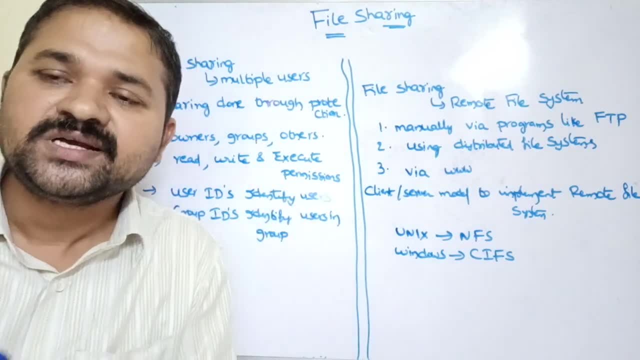 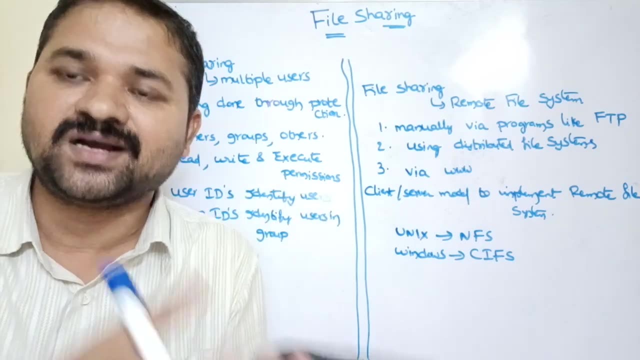 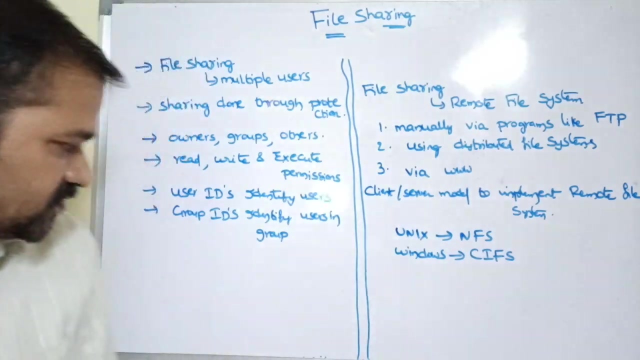 checks whether that person has that permission or not. So if that person has the following permission, then the corresponding permission will be granted, Suppose if the person has not having that permission so that command won't be executed by the operating system. So, with the help of 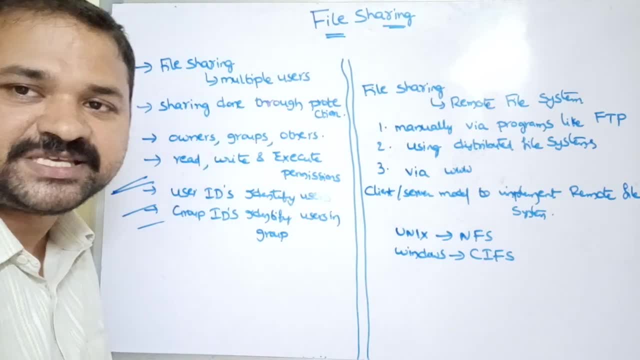 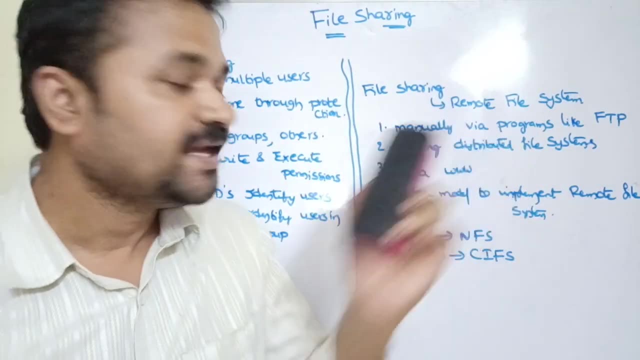 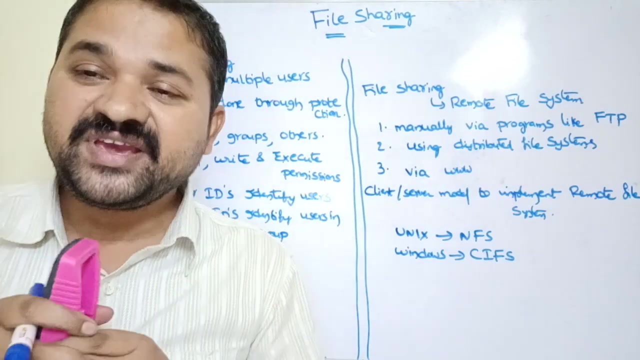 these user ids and group ids, operating system can share the file among multiple users. Now let's see how sharing can be implemented in a remote file system. So we know what is a remote file system. Nowadays, with the help of networking, we can connect several computers that are located at different portions of the world- One computer. 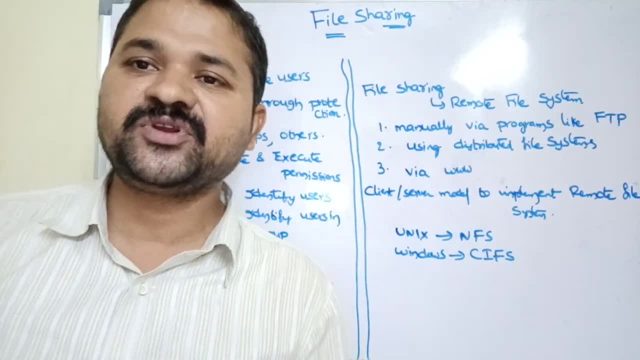 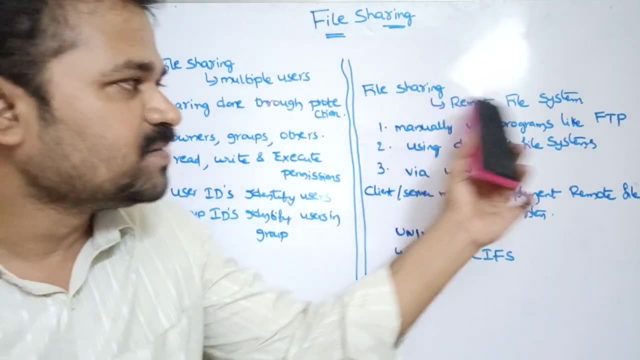 may be in India, another computer may be in US, next computer may be in UK. So we can connect all those computers with the help of the computer networking. That is nothing but remote file system. So remote file system means the corresponding file is. 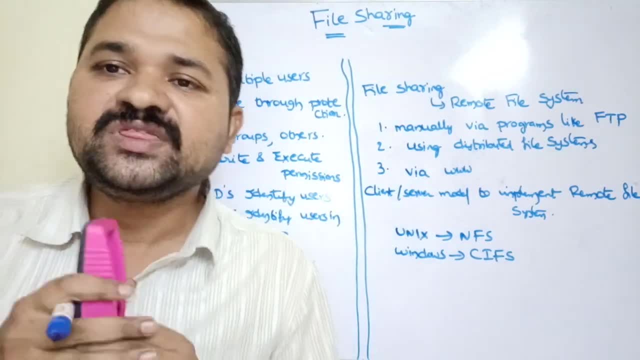 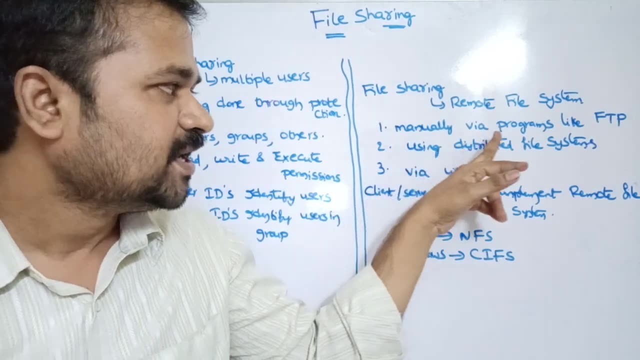 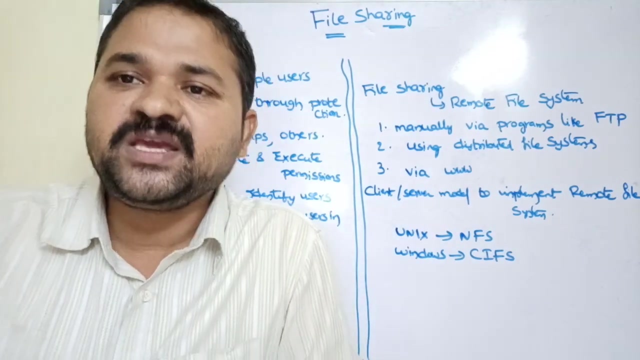 available in a remote mission, a server. So in that situation, how we can implement file sharing? So for that we have three approaches. The first approach is manually, via programs like FTP. FTP stands for file transfer protocol, So by using FTP we can transfer a file from. 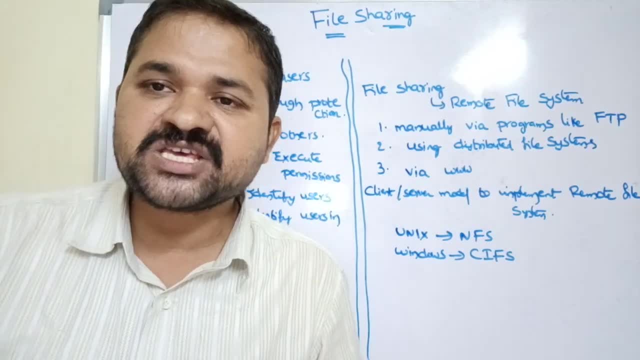 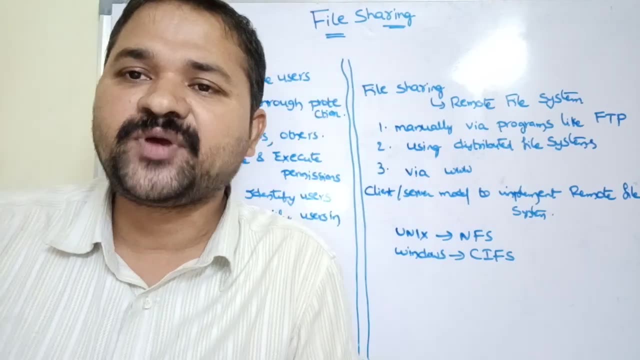 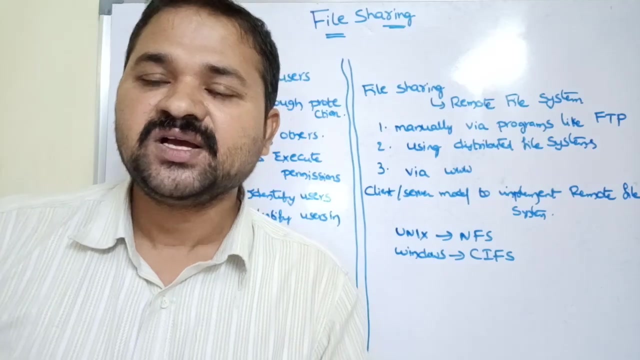 one mission to the another mission. So in the client mission we execute FTP, So that program sends a request to the server. So server executes the corresponding program and it provides the corresponding file to the client mission. And the second approach is distributed file system. So distributed file system means the file can be distributed among 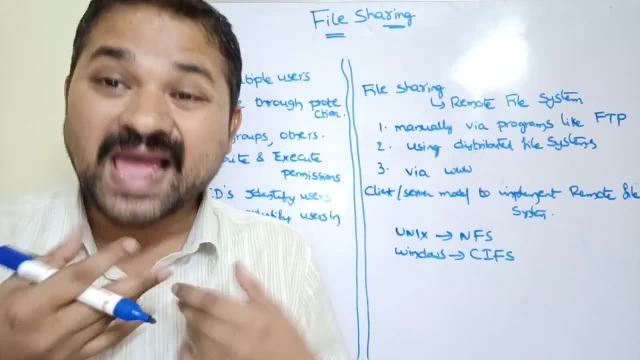 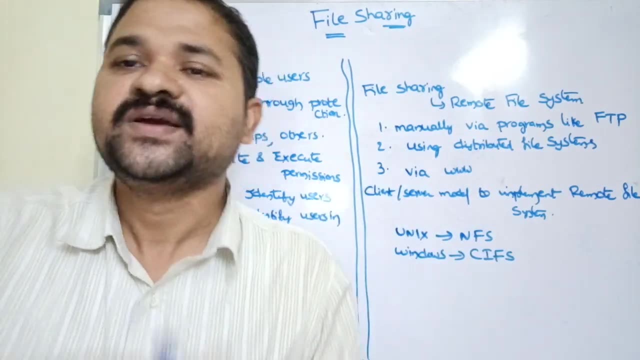 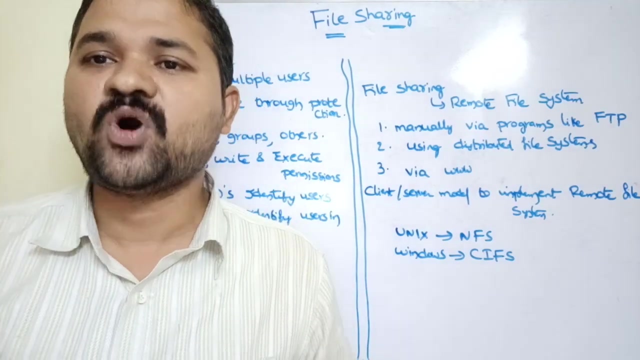 the systems that are connected So that the client mission can use that file as it is available in the local mission. But actually that file is available in some other server, So that is known as distributed file system. So the corresponding file is distributed among 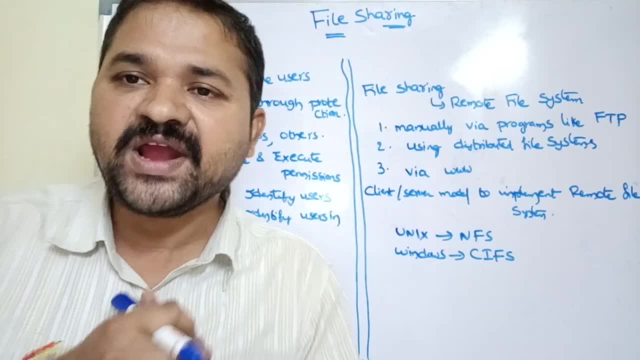 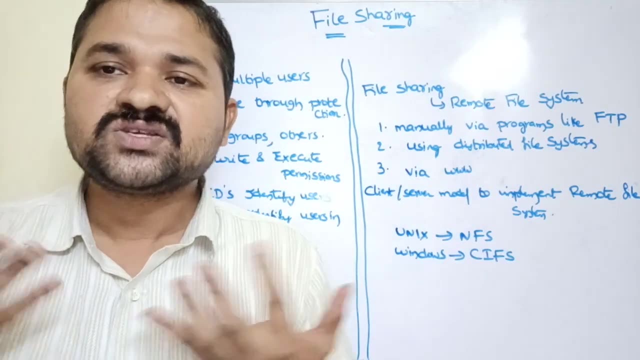 several systems in the network And the next one is via worldwide web. So with the help of a browser we can type some URL so that request will be sent to the server. So server process the corresponding request and it sends the corresponding file to the client. 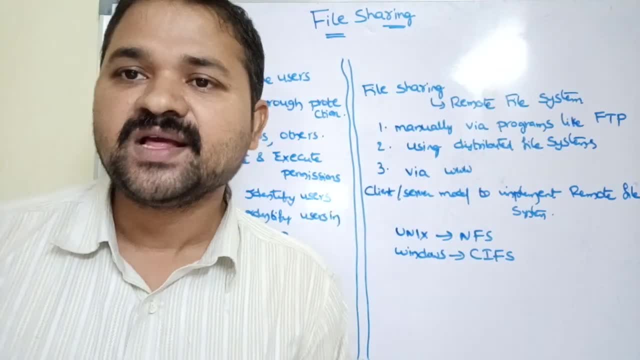 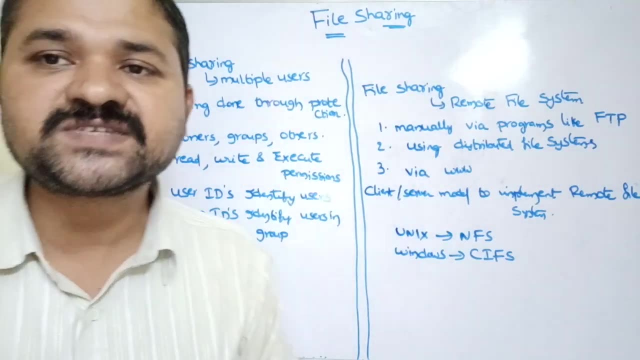 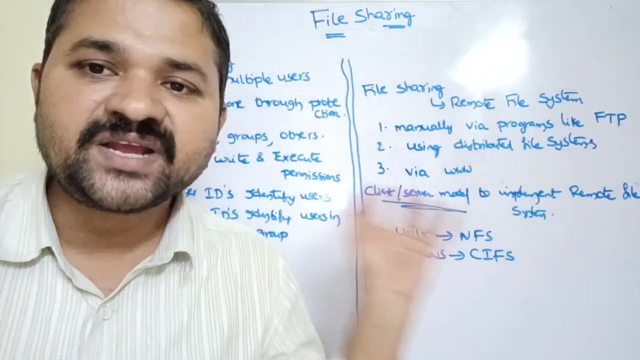 So by using these three approaches, we can implement the remote file system. So the first approach is file transfer protocol, The second approach is distributed file system and the third one is via worldwide web. So in order to implement the remote file system, we use this client server model. So here we are using client server model. 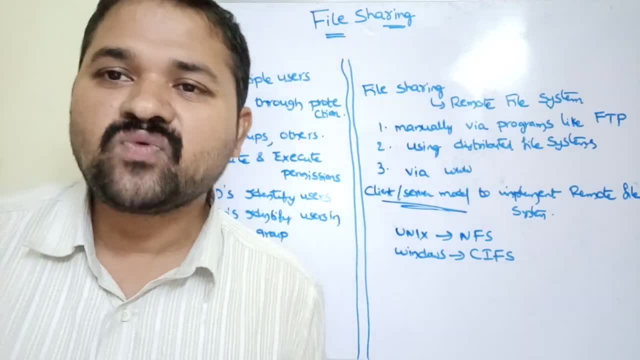 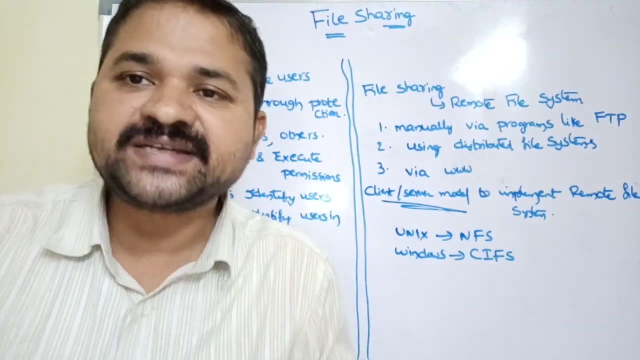 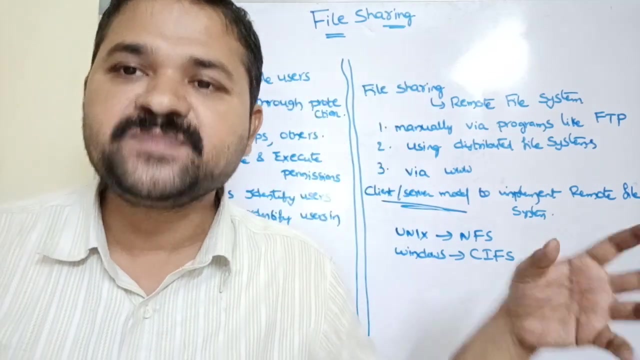 in order to implement a remote file system. So we know what is a client server model. So client sends a request to the server, So server process that request and provides the corresponding response to the client mission. A server can handle multiple requests that are sent by the multiple 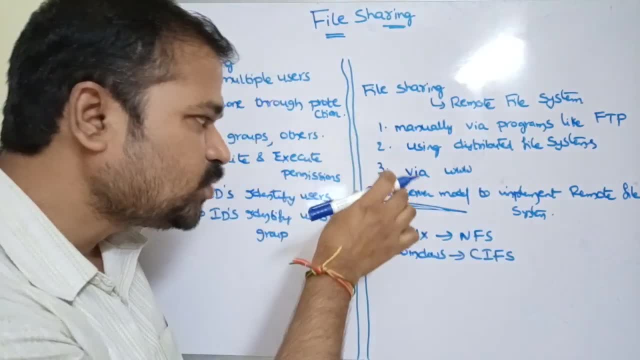 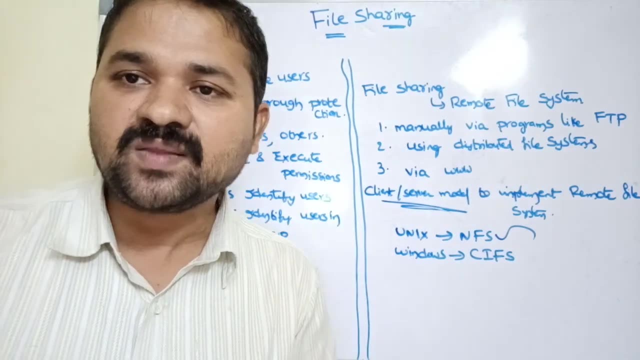 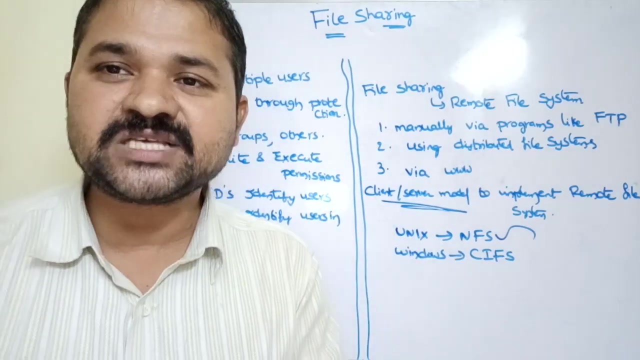 requests. If you take Unix, then in order to implement client server model, we use NFS protocol. NFS stands for network file system protocol. So by using network file system protocol we can implement client server model in Unix operating system or Linux operating system, Whereas if you 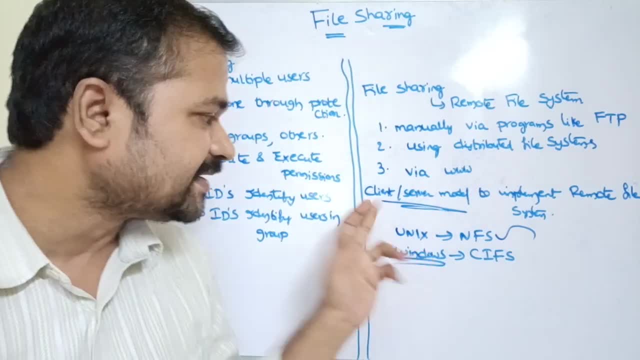 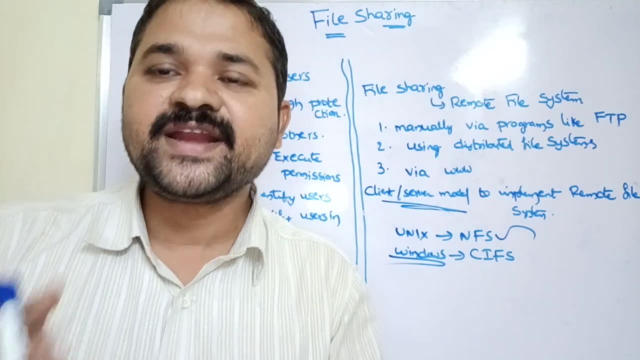 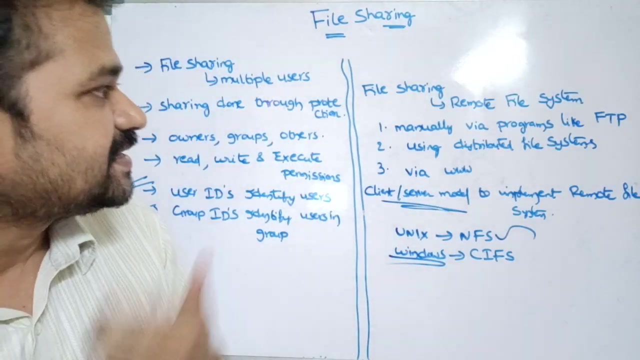 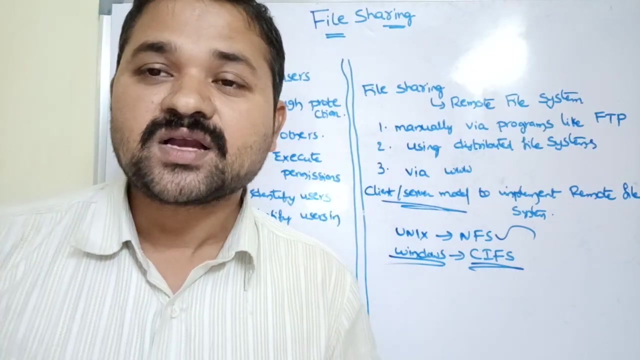 take Windows operating system, then in order to implement the client server model, we use CIFS protocol. CIFS stands for common internet file system protocol. So in Windows operating system, in order to implement the client server architecture or the client server model, we use CIFS. CIFS stands for common internet file system. So, with the help of